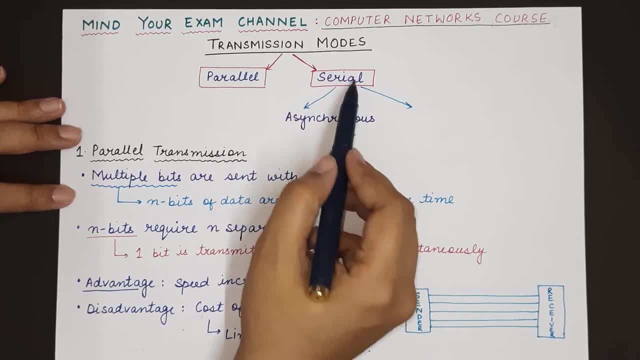 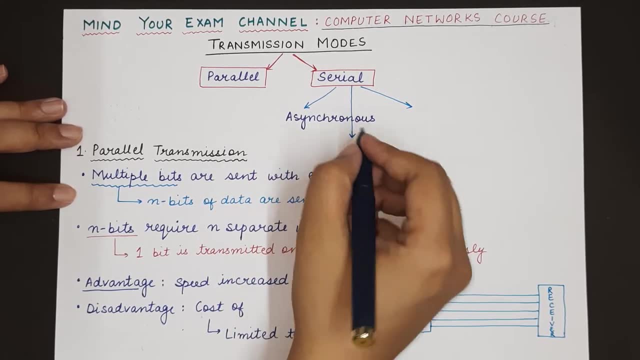 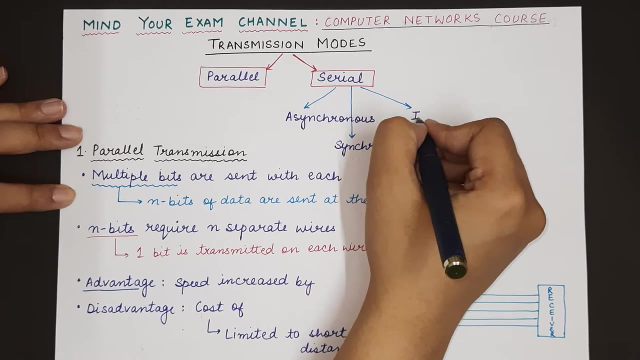 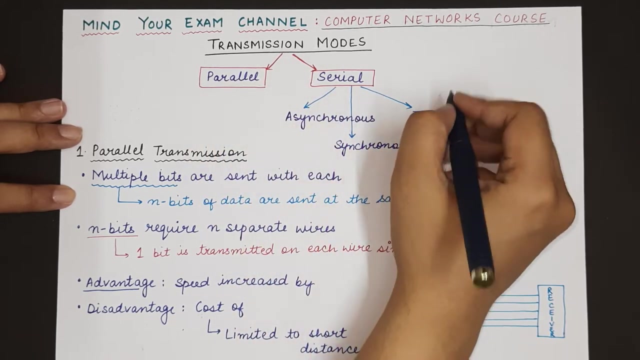 transmission mode is and what are the types of serial transmission? So there are three types of serial transmission modes: First is asynchronous, the second is synchronous and the third one is isosynchronous. So we will be studying all the three of them in detail, along with the parallel transmission mode, also isosynchronous, So parallel transmission. 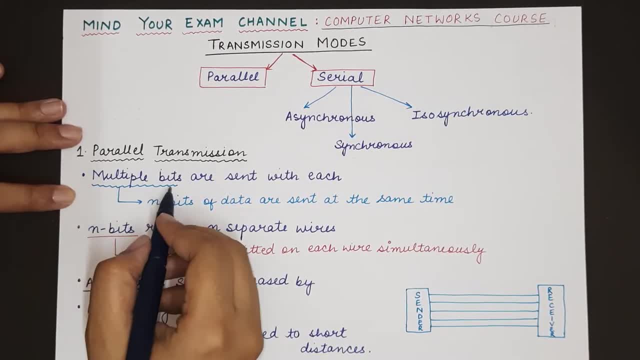 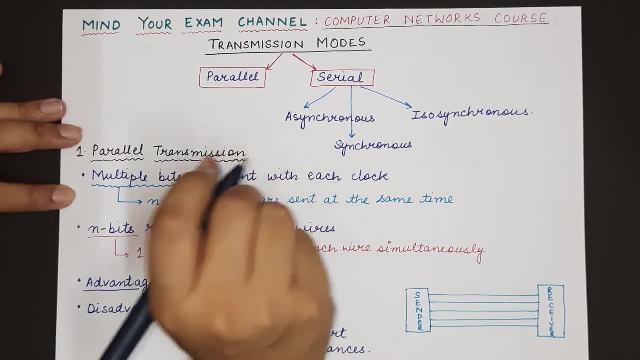 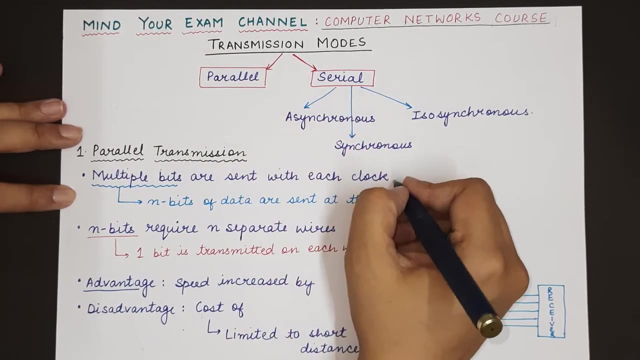 mode. So parallel transmission mode, basically means that multiple bits are sent with each clock tick. That means at each point whenever the sender is sending some data. then multiple bits will be sent at the same time with each clock tick. Now, multiple bits means that if 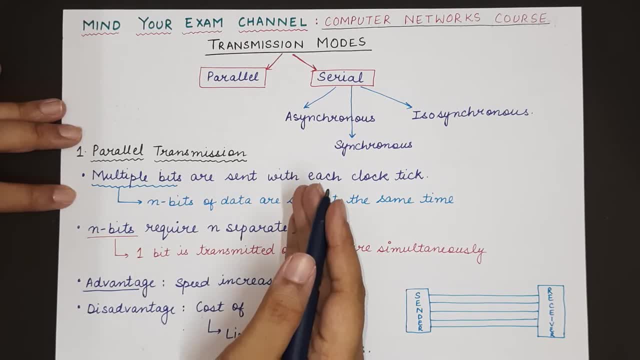 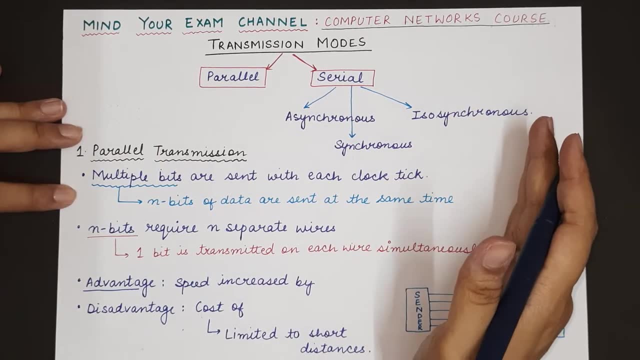 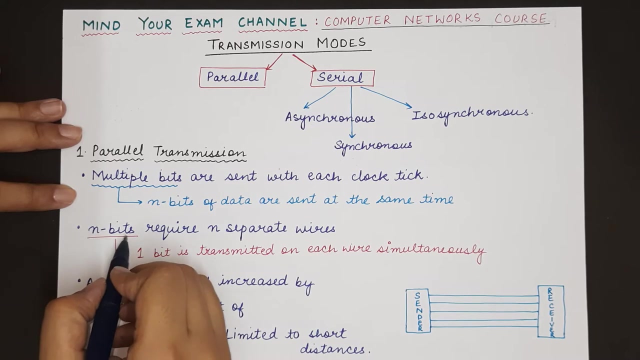 there are n number of bits that are being transmitted by the sender, then each of these n bits will be sent at the same time. So this is possible when we have multiple channels. that means for each of the end bits we require a separate wire that can carry the bits separately, So one bit can be transmitted. 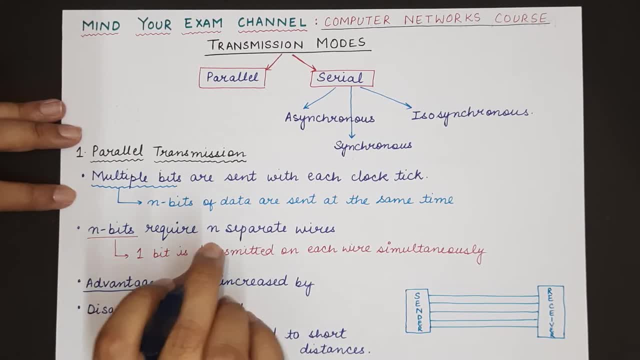 at one moment, I know, in a wire. okay, So if we have a physical wire that is used for transmission, that at then, at any moment, we can only transmit one bit at a time. But if we have to transmit multiple bits at the same time, then we need multiple wires. okay, So n bits will require n separate wires, such that 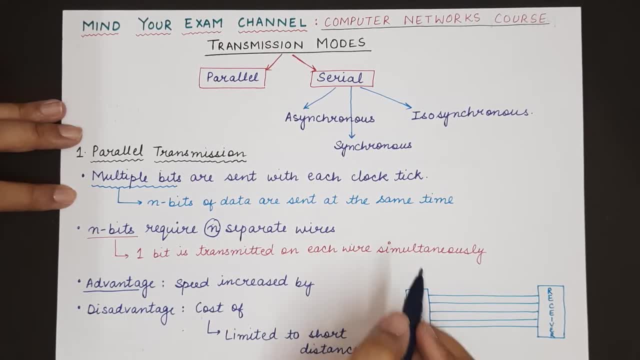 one bit will be transmitted on each wire and each of these bits will then travel simultaneously. So if this is a sender who wants to send five bits in parallel, then the sender will maintain five different channels of communication. That means he will maintain five different wires. 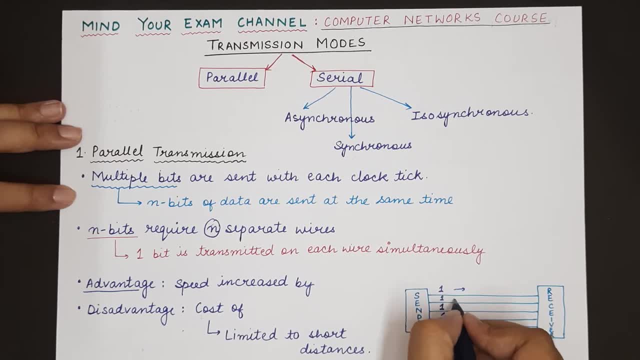 such that at every moment he will send five different bits. The bits can be different. it can be 0,, 1, 0, any format, any combination can be formed. but all these bits will be carried separately on each wire and they will travel simultaneously and reach the receiver.